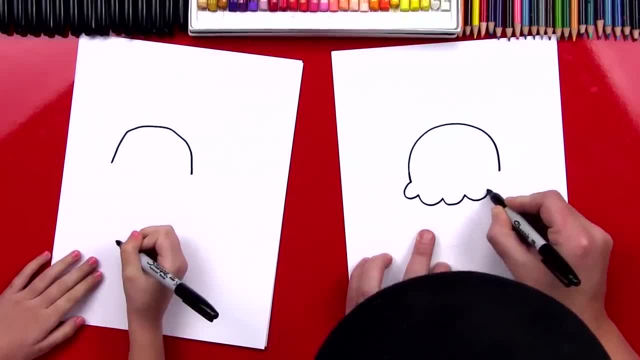 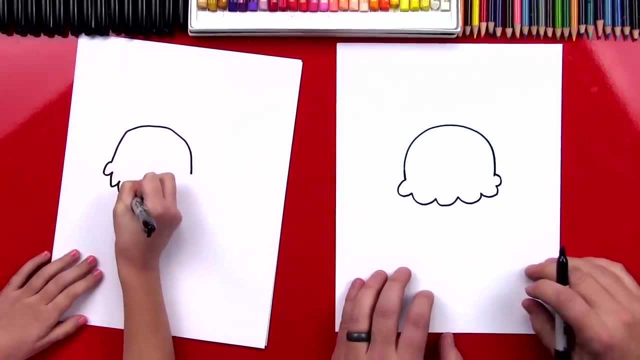 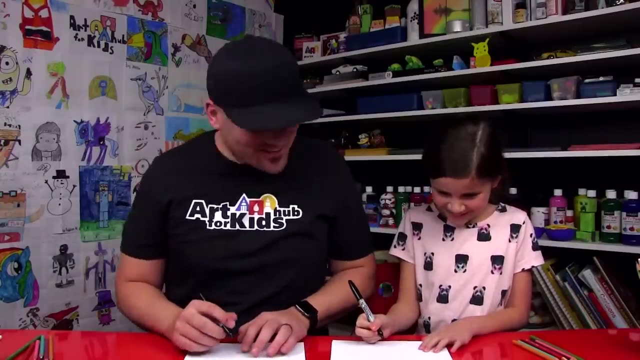 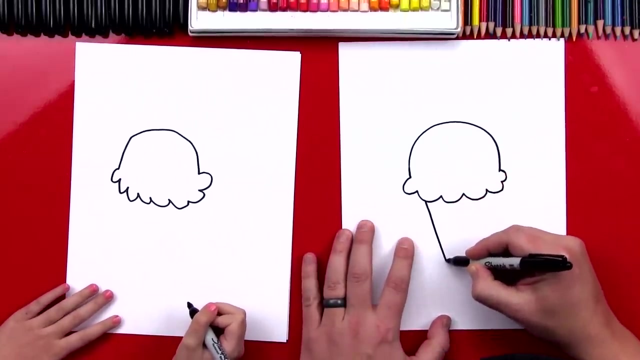 too. We're going to go all the way over to the other side. Okay, I like it Was that fun, Yeah, Okay, good, Now we're going to draw the cone. So we're going to draw a line that comes down and we're going to make a V shape and then it's going to come back. 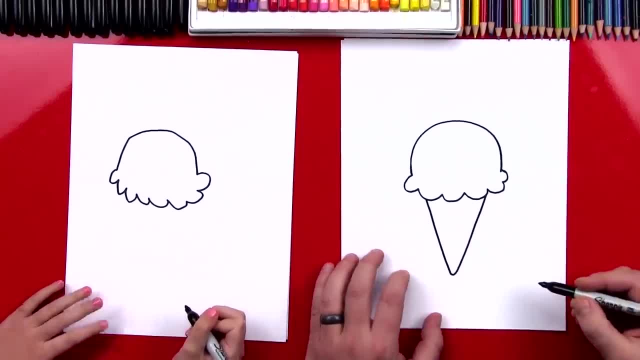 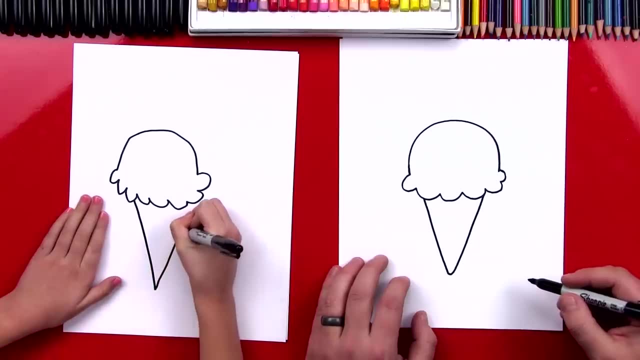 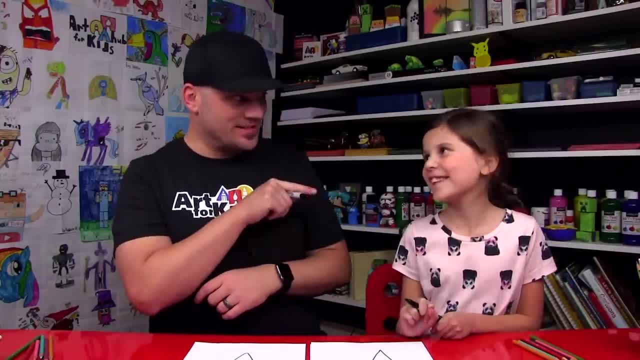 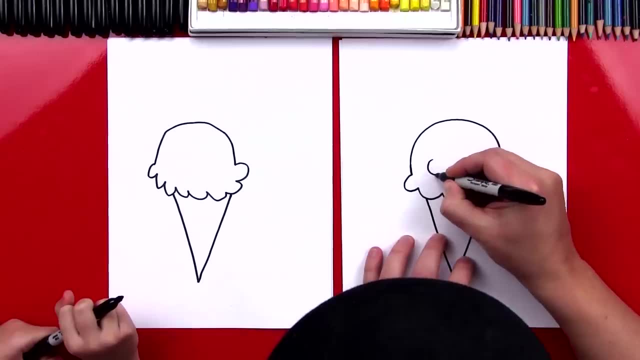 details. right, Yeah, What should we add? A face, A funny face? Yeah, Okay, let's do it. We're gonna add a funny face right to the ice cream scoop. We're gonna draw a circle right here. We're gonna. 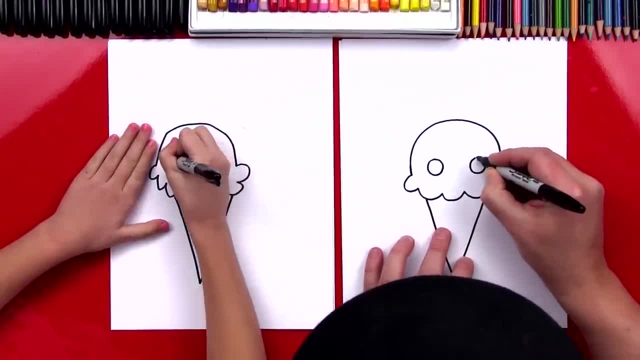 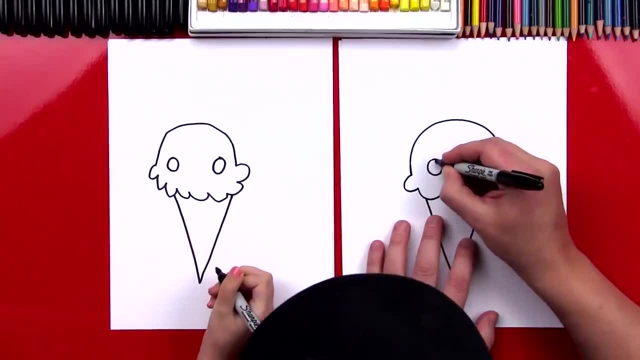 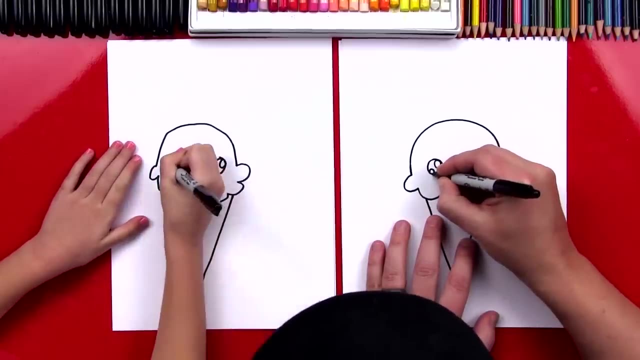 draw one right here and I'm gonna draw another one way over here. Yes, and then let's draw those small circles inside in the top right on both circles, and then we're gonna draw a little smaller circles down the bottom left. Then we're gonna color in the big circle and leave those little. 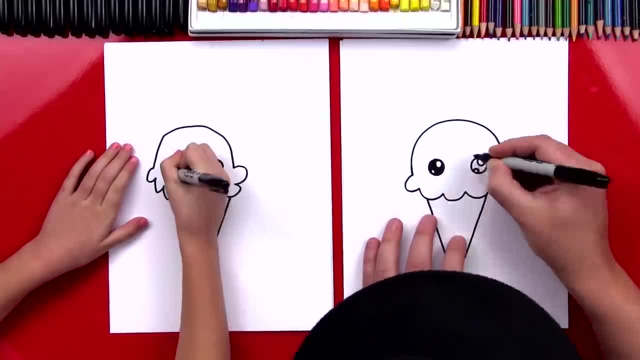 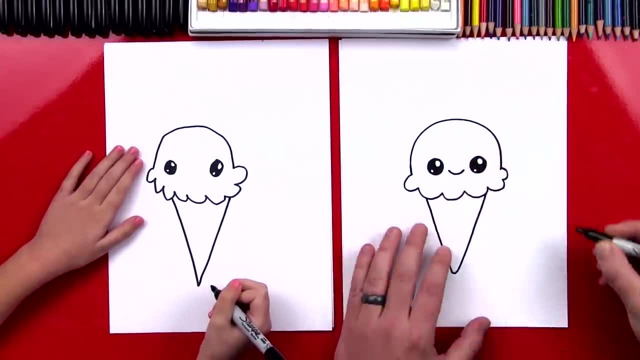 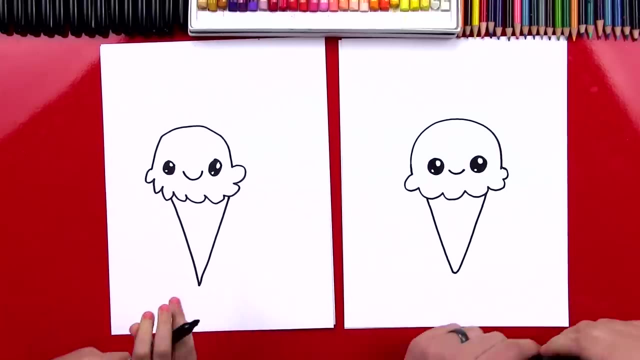 circles white. Okay, Should we make our ice cream happy? Yeah, All right, let's draw a smile right in between his eyes or her eyes. We did it, Haz. Okay, now let's put our markers off to the side. and what should we do next? Color, Yes, let's color our ice cream cones. and this part we're gonna fast forward. 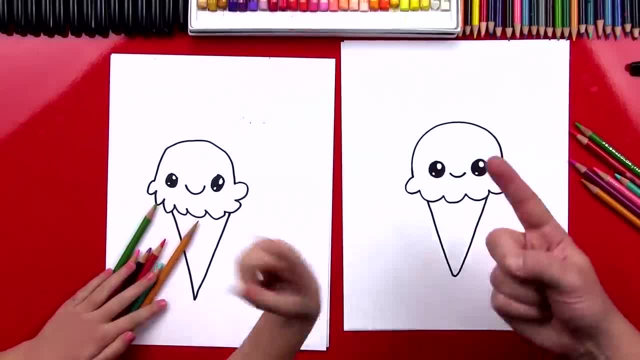 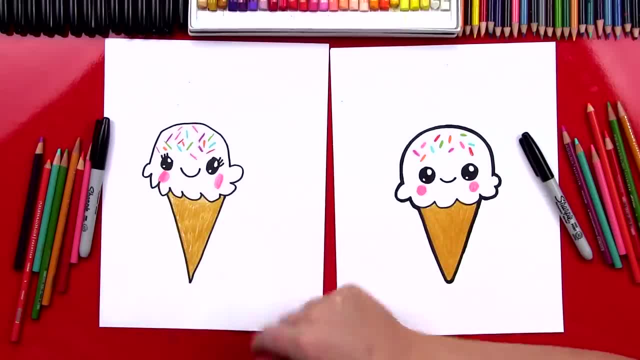 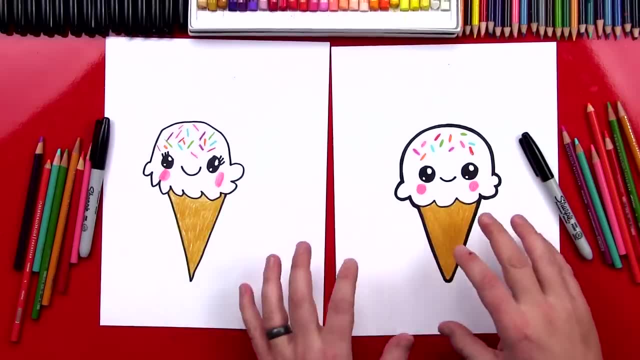 Hadley, you did awesome. Give me five. Did you have fun? Yeah, What was your favorite part? Um, the eyelashes, The eyelashes. I love the extra details you added. Now you guys at home can pause the video to match the coloring that we did, or you could use your imagination and add your own. 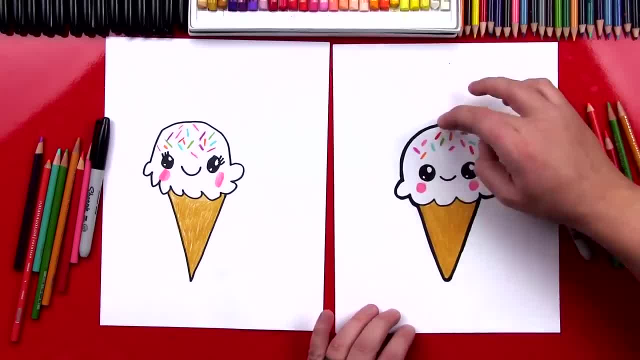 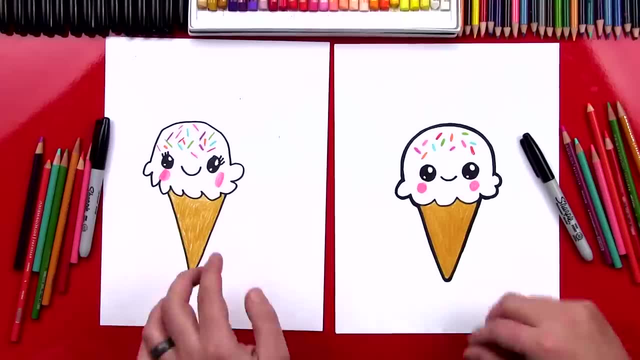 details. Maybe you add more scoops on top of it. Maybe you add more scoops on top of it. Maybe you add more scoops on top of it. Maybe you can even add a cherry, Yeah, Yeah, you could do different flavored ice cream too. Yes, Are you getting hungry? Now? it's okay that our drawings look a.